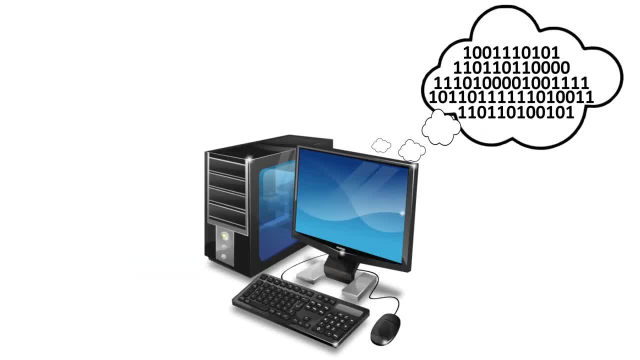 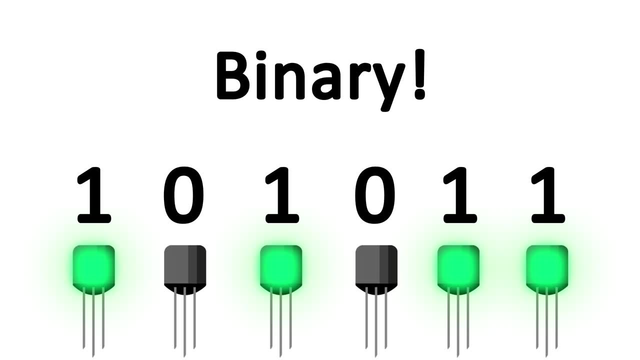 In the video I made on binary I explained why it is that computers use 1s and 0s to think. The 1s and 0s represent the state of a single electrical cell inside the computer, which can be one of two states. But is this the only way of doing it or are there other options? 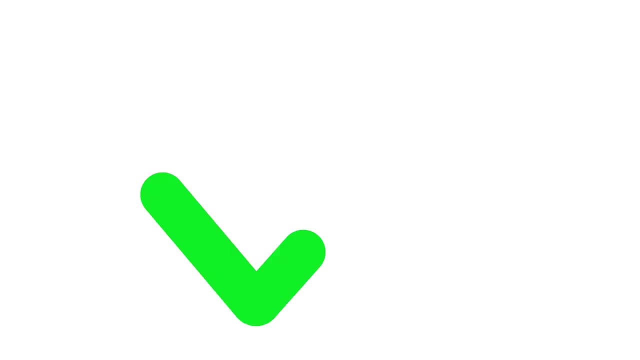 that let us work with more than just two states. Well, actually, yes, there are, And in the early years of computer engineering, people experimented with computers that could use base 3,, base 8,, base 10, and even base 16.. So why were these methods abandoned? in favor? 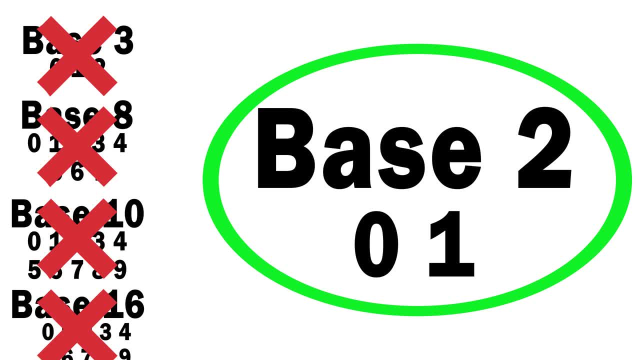 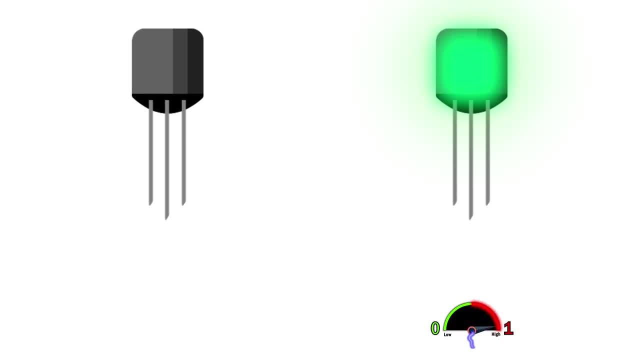 of binary. If you want to know, then this video is just for you. So to clarify one thing: when we refer to a transistor being on or off, what we really mean is that it's either a high charge or low charge, respectively. An on cell has a. 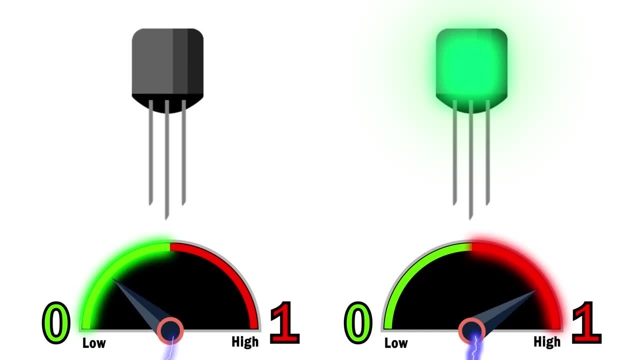 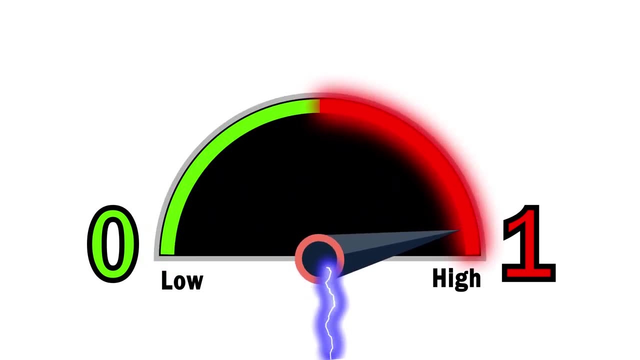 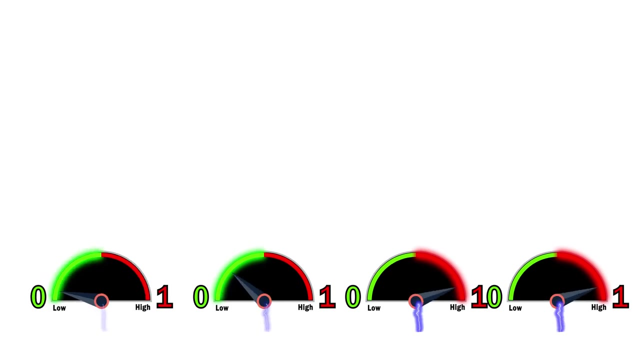 very high amount of electricity stored in it or moving through it, while an off cell has a low amount. These states determine whether or not a single cell is a single cell or a single cell is a single cell. So if a computer can read and write data to these cells by sensing or storing different 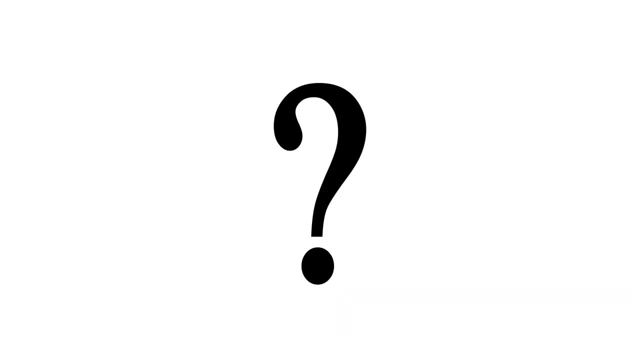 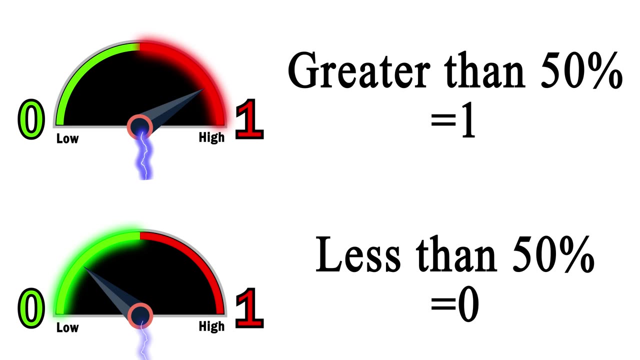 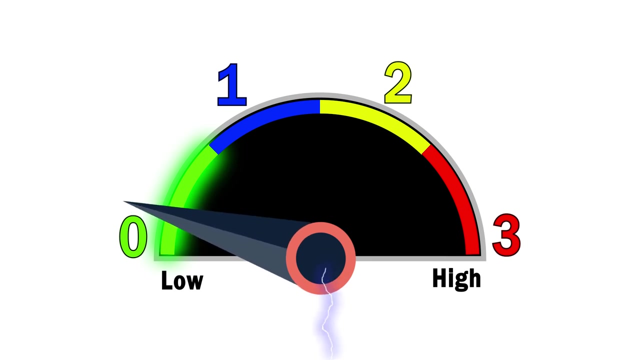 amounts of electrical charge in each one. why can't we get more specific with them? What if, instead of less than 50% charge being a 0 and above 50% charge being a 1, we divided it into four segments like this: Now, 0 to 25% charge could be a 0, 25 to 50%. 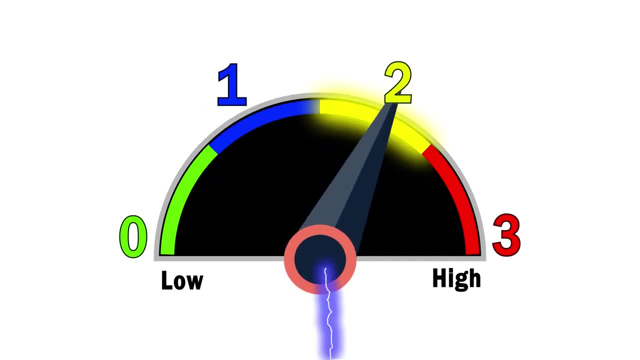 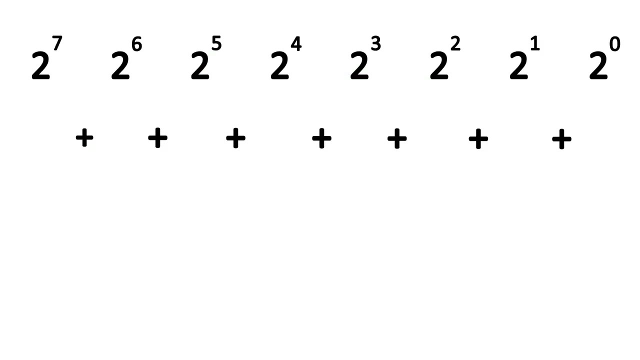 could be a 1,, 50 to 75% could be a 2, and 75 to 100% could be a 3.. With this method, each individual cell could have four states, meaning that each byte of data could be a number designed around base 4, instead of around base 2.. Where a byte 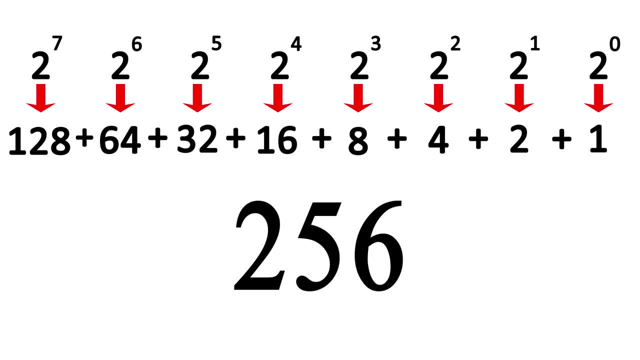 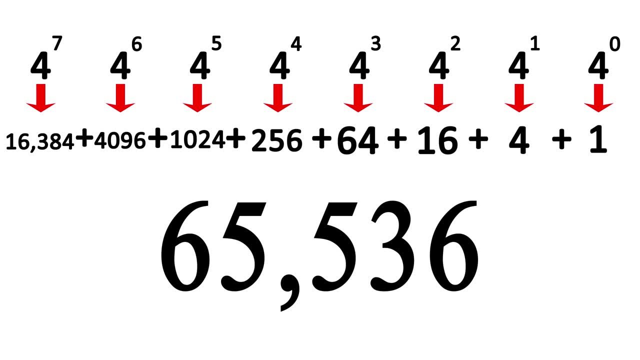 of 8 transistors could have 256 values with base 2, our new system could let us have 65,536 values with base 4.. Way better, right, Better, right. Better yet, what if each cell could represent 8 or 10 or 16 different states by making the 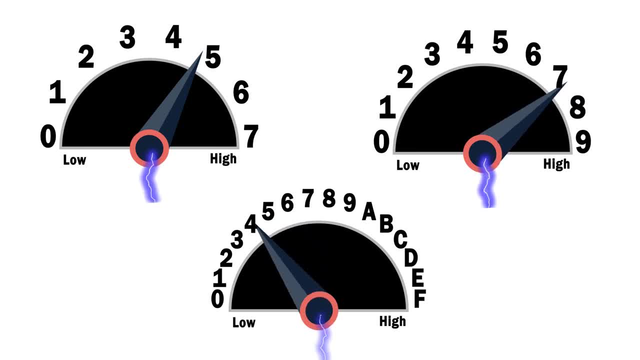 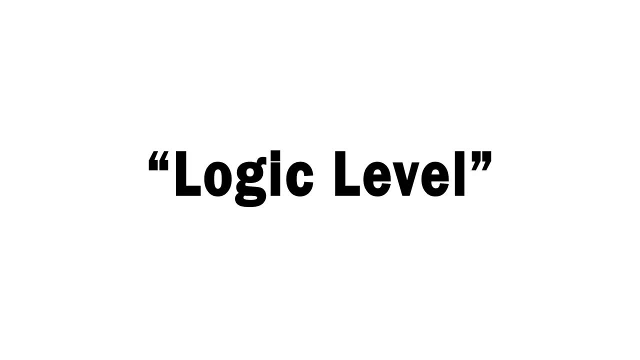 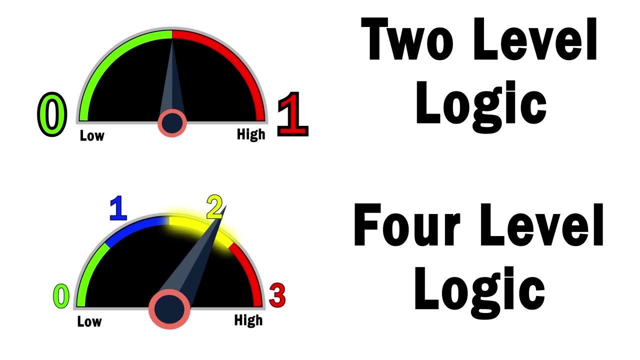 bit even more precise. Well, as mentioned above, these methods were experimented with. The amount of states a single cell of information can hold is referred to as a logic level. Binary is called 2-level logic, and the one I just described would be known as 4-level logic. 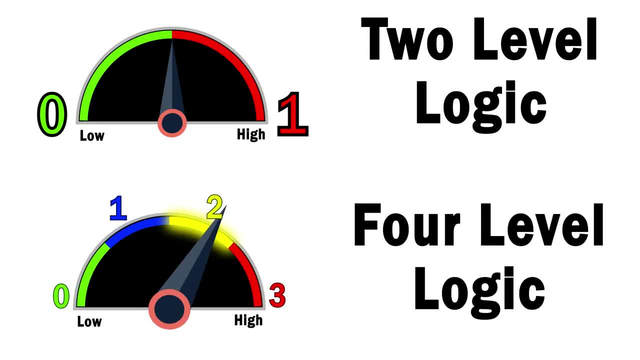 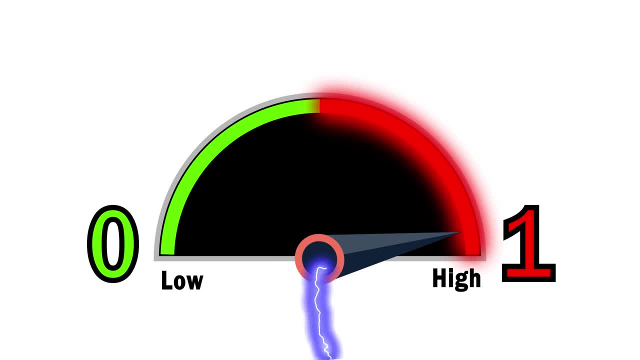 The fundamental problem with using logic levels greater than 2 to represent numbers is reliability. While computers are really good at storing and reading the electricity in each cell, the exact voltage tends to fluctuate a little bit. Take a look here: The sort of natural 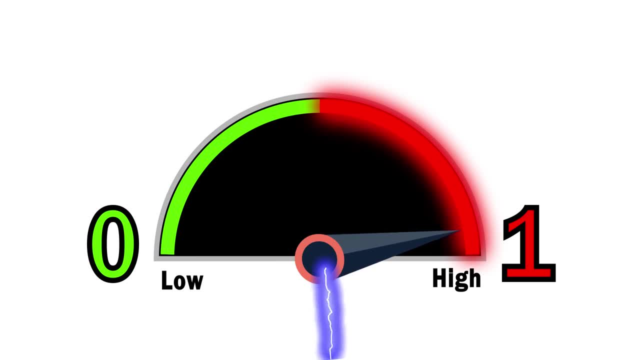 fluctuation of electricity means that the level of voltage in this cell of data wobbles off by, let's say, 20 percentage points. Even if things get really bad, like 40% off, we have a lot of leeway on either side For an on state. we try to keep it at 100%. but if it falls every now and then, it's still above 50% and we don't want to lose it. So let's take a look at how we can keep it at 100%. but if it falls every now and then, it's still above 50% and we don't want to lose it. So let's take a look at how we can keep. it at 100%, but if it falls every now and then, it's still above 50% and we don't want to lose it. So let's take a look at how we can keep it at 100%. but if it falls every now and then, it's still above 50% and we don't want to lose it, So let's take a look at how we can keep it at 100%. but if it falls every now and then, it's still above 50% and we don't want to lose it, So let's take a look at how we can keep. it at 100%, but if it falls every now and then, it's still above 50% and we don't want to lose it. So let's take a look at how we can keep it at 100%. but if it falls every now and then, it's still above 50% and we don't 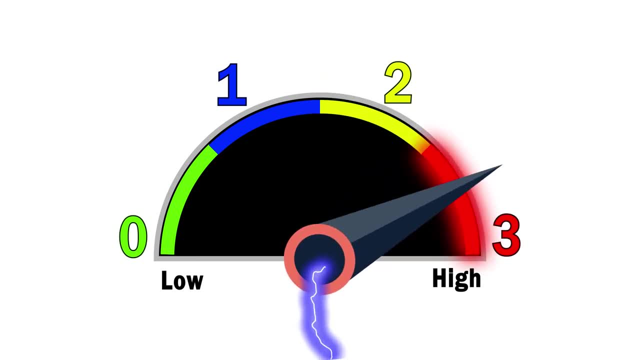 want to lose it. So let's take a look at how we can keep of states in each cell. the more specific this voltage has to be and, by extension, the more likely it is to be wrong. It's especially difficult to try to balance the voltage in the middle, where 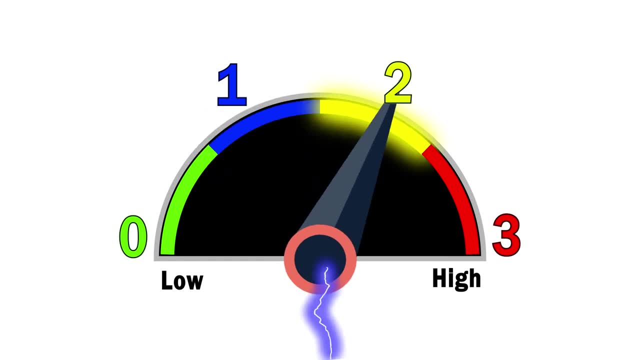 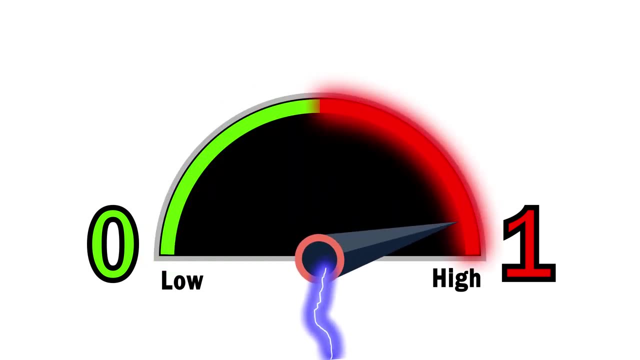 it can't be too high or too low When we only have two states. for off, we can keep it as low as possible, and for high, we can keep it as high as possible. We don't really have to worry about overshooting in either direction. This is the primary reason we settled on base 2.. If a single 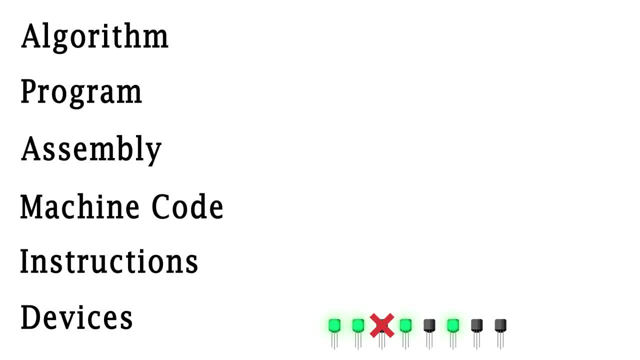 unit of information is wrong, then the entire number represented by the byte is wrong. And if your byte is wrong, the data is wrong, your code won't work and your instructions will be misread. Everything just falls apart. It only takes one bit of data being wrong for this to